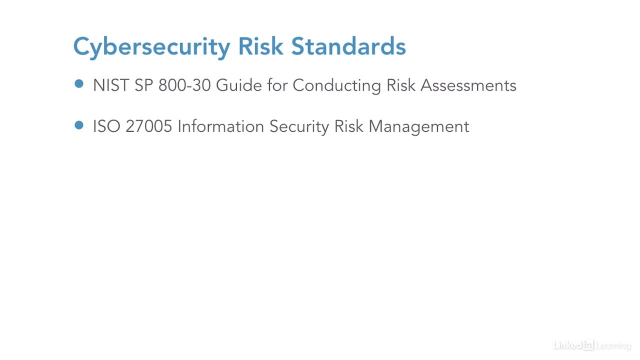 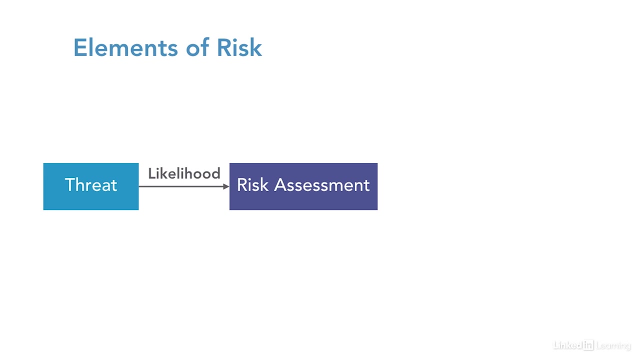 Information Security: Risk Management publication. While there are minor terminology differences, the intent of both documents is the same. Risk starts with a threat event, which must be analyzed to determine the likelihood that the event will occur. This is done by considering the likely threat actors, their capabilities and their resources. 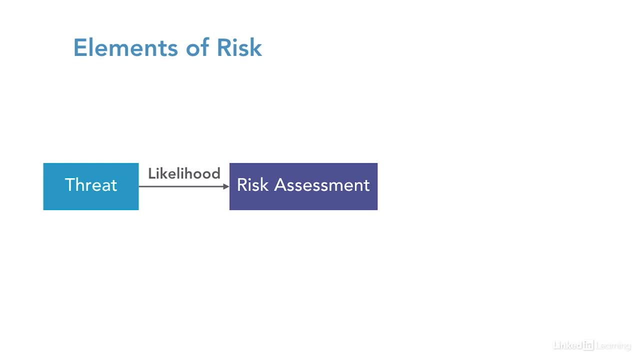 The intent or motivation needs to be considered. What is it that drives this threat actor to want to mount an attack? An attacker will only attack if the results outweigh the cost of attacking, and that depends on the value of the target to the threat actor. This could be financial gain. 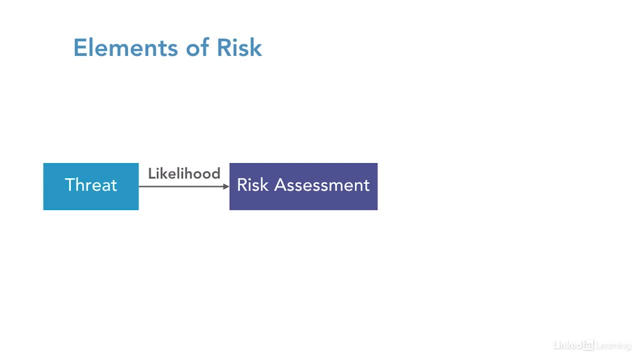 obtaining intelligence, disrupting services or just peer recognition. The next thing to think about is the set of vulnerabilities in the information and processing assets, The databases, workstations, servers and networks which this event can exploit to cause damage. For instance, a data center in the basement of. 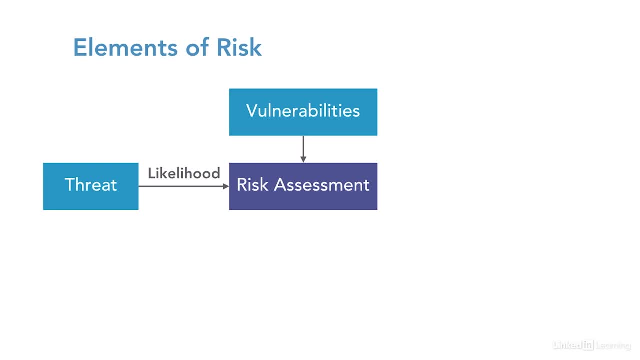 a building may be vulnerable to a flood event. A website may have a software vulnerability which can be exploited. A server without an uninterruptible power supply would be vulnerable to a power outage. However, not all vulnerabilities are equal. A flood may be. 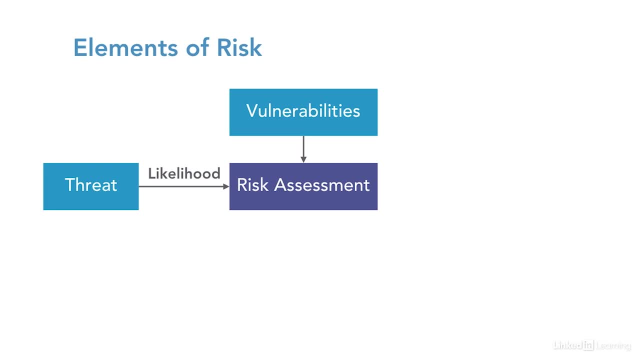 catastrophic. A data center in the basement of a building may be vulnerable to a flood event, With the whole data center out of action for weeks, whereas an attack which exploits a website floor may just be a nuisance. The next thing to consider is the impact to the business of an event. 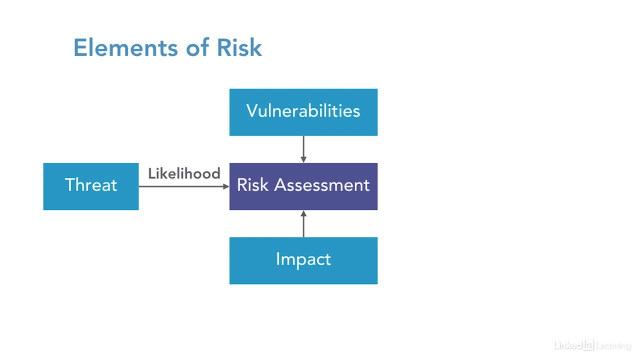 This is typically done by carrying out a business impact assessment to determine what systems will be affected, how this flows on to business processes and the cost of service degradation or failure to meet critical levels of performance. Being able to describe a security event as a 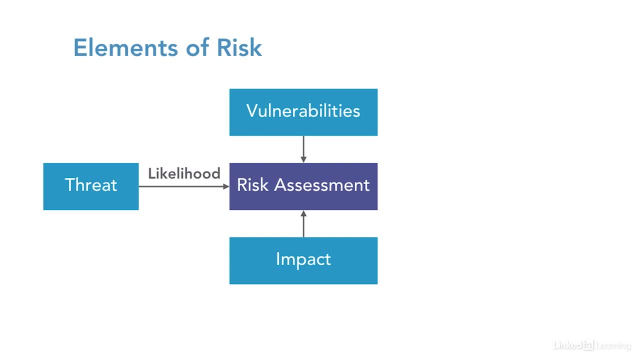 business impact can be a big part of the process. The next thing to consider is the impact to the business of an event. This can be done to determine our confidence and choice and the equal institutional tension that we may experience. But there is still room for improvement. 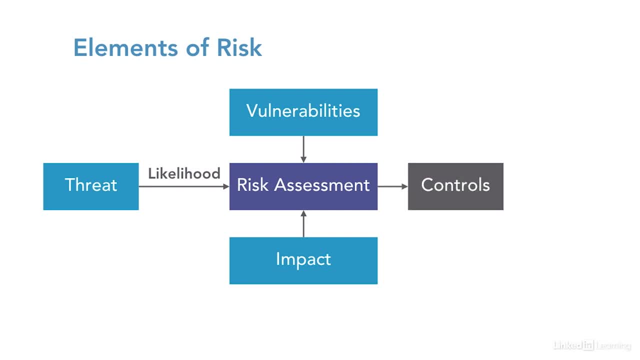 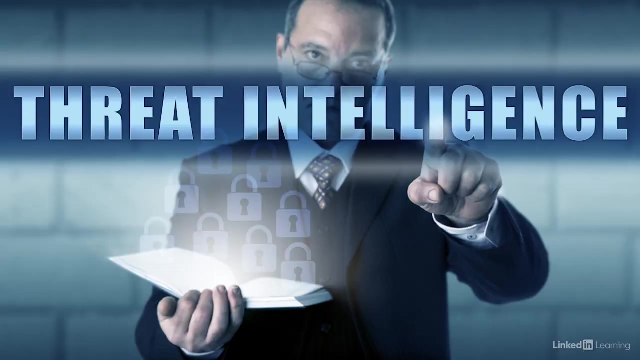 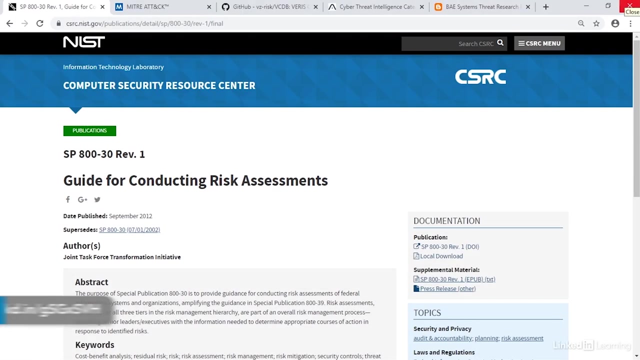 A мой detail statement is a performance statement that helps water sewer use. A useful catalogue of threats can be found at Appendix E to the NIST Special Publication SP830.. This catalogue provides representative examples of threat events expressed as tactics, techniques and procedures or TTPs. 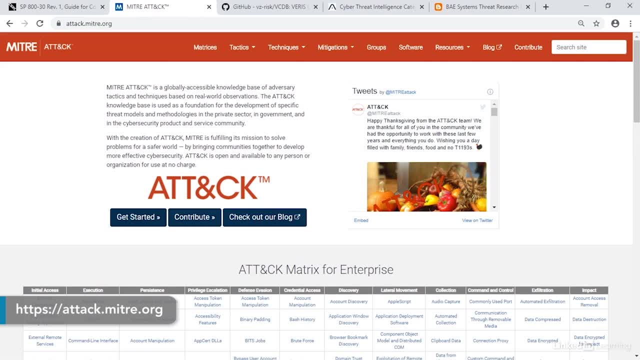 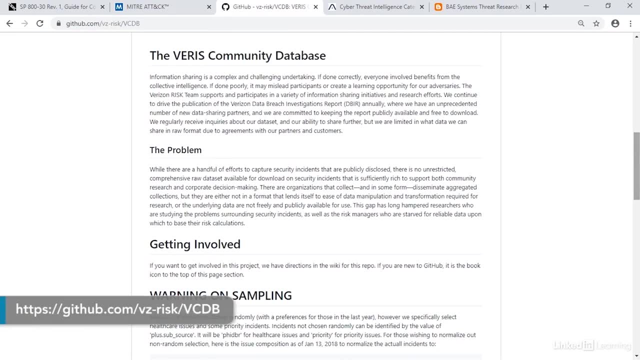 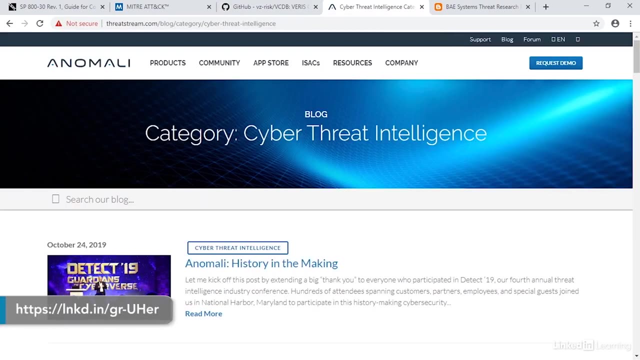 Another very useful source of TTPs is the MITRE ATT&CK site, which is used in MITRE's Cybersecurity Resiliency Framework. VERIS provides an open community threat database which can be used to support risk analysis. ThreatStream offers an open-source cyberintelligence blog which reports on contemporary activities and threat actors. 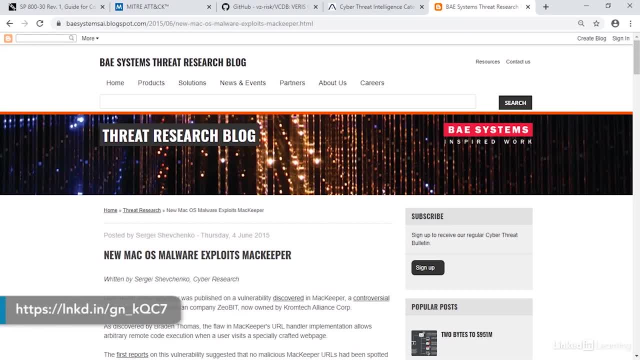 There are a number of good sources of specific threat reports, which provide detailed information on threat actors, threat techniques and target vulnerabilities. Here we see a report from BAE Systems' Applied Intelligence On a vulnerable application called MacKeeper that can be exploited to attack MacOS systems. 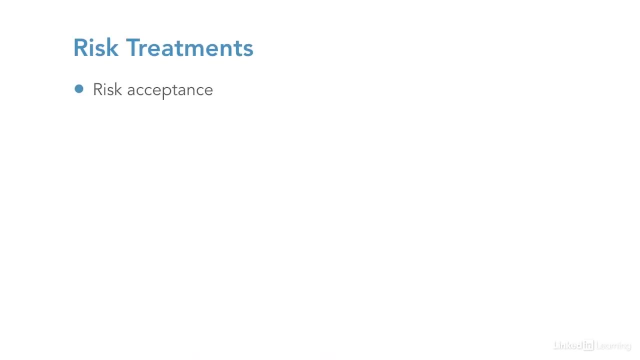 There are four possible treatments once an assessment has identified the risk. Risk acceptance, where the risk is within the business' appetite. Risk avoidance, where it's better to stop doing that line of business than take the risk. Risk transfer, where a third party takes the risk, such as insurance to cover risk should it eventually occur. 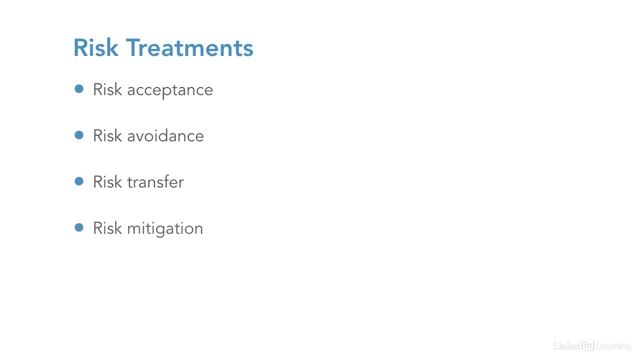 And risk mitigation, where controls are implemented to reduce risk. Risk mitigation and the protection of business outcomes, which they provide, means implementing controls in the form of cybersecurity policies, procedures and technical solutions. There are four key types of control that can be applied, and it's generally recommended that two or more are used together to achieve defense in depth. 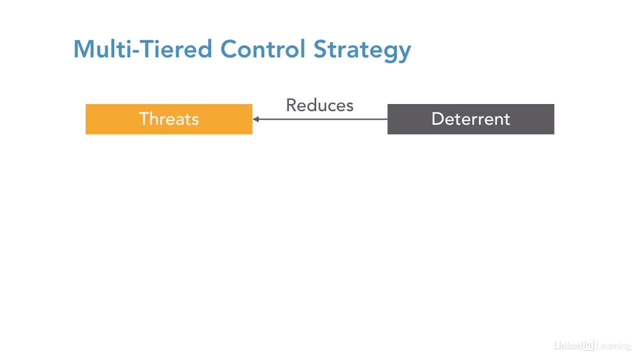 The first is deterrent controls. These reduce the threat. An example of this is incarceration, which deters would-be criminals from carrying out their attacks. Preventative controls are designed to stop the attack from succeeding by not allowing it to get at an asset to exploit a vulnerability.